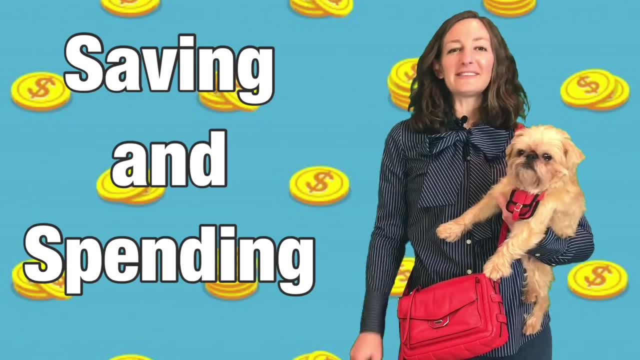 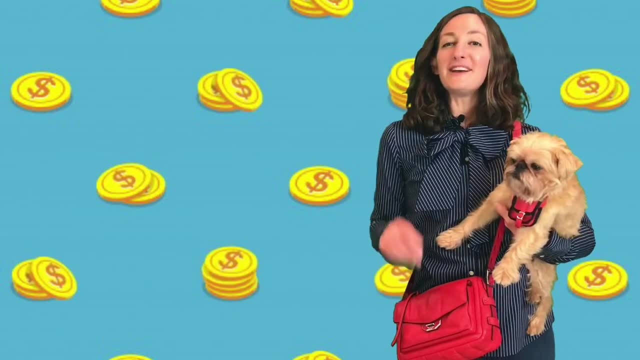 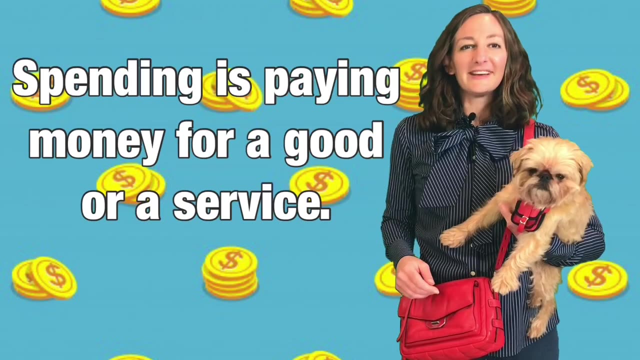 Hi everyone, Ms Dahlman and Lucy here, and let's talk about money. You know moolah, dough paper. People can earn money through a job, or maybe you even earn money through an allowance by doing chores at home. When you spend, you are paying money for a good or a service. 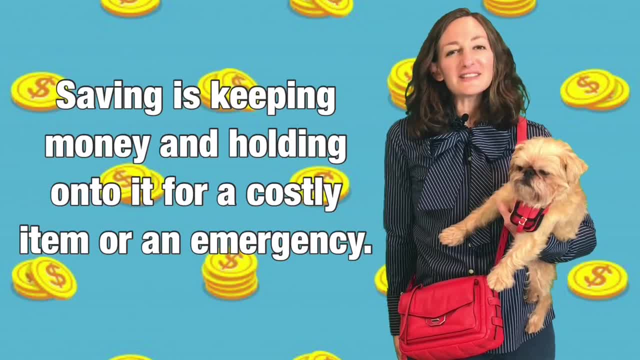 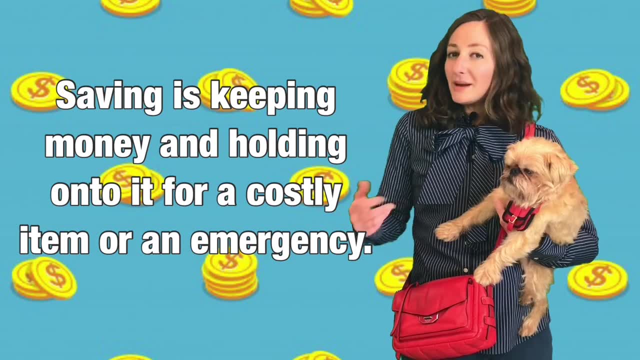 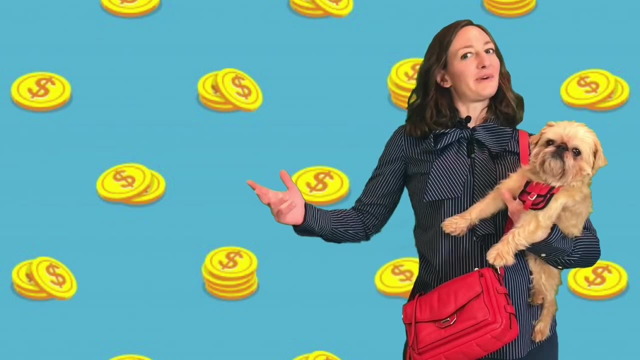 Saving. Well, that's just the opposite: Keeping money and using it for later, for something that costs a little more, or maybe in an emergency. You know it doesn't make much sense to spend all your money in one place. so let's see what Lucy and our other friend, Milo, do when. 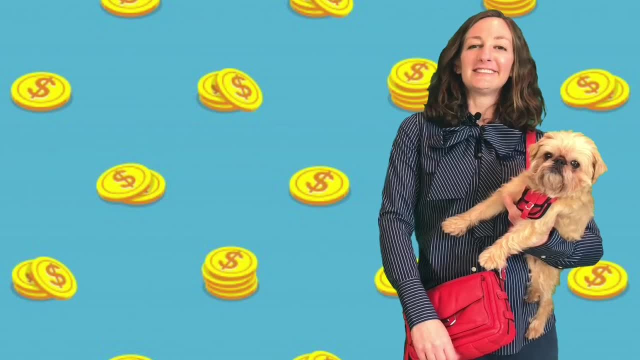 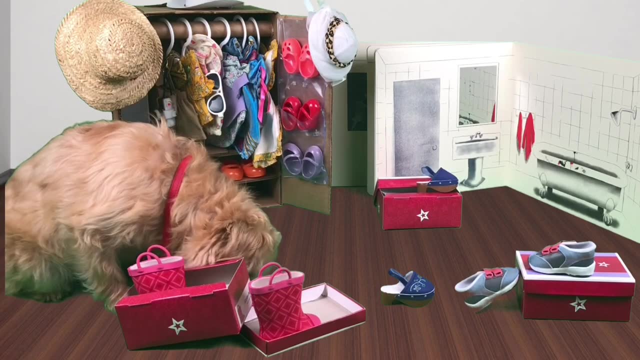 it comes to spending and saving money. Enjoy Now. Lucy is a very good person. She's a very good person. She's a very good person. She is a spender. Although she has a closet full of shoes, she just bought three more. 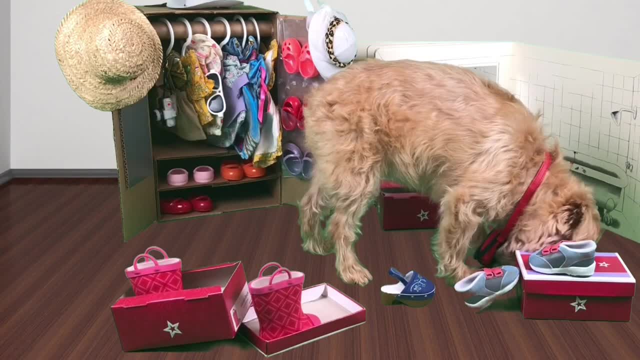 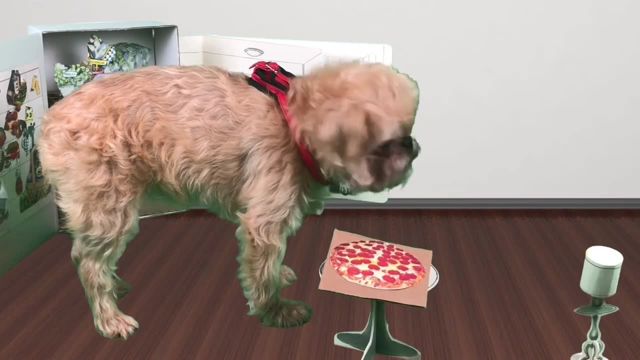 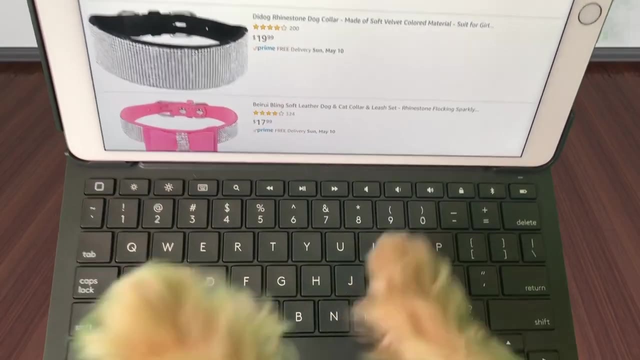 pairs Here. Lucy has spent money on ordering pizza, even though she has a fridge full of food. Shopping online for things that you don't have to have is a good way to spend money. She's a good person. She's a good person. She's a good person. She's a good. 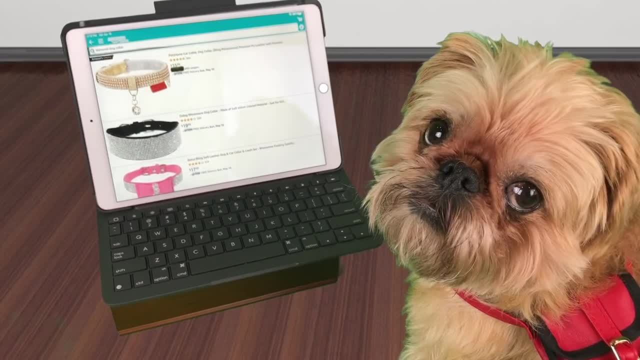 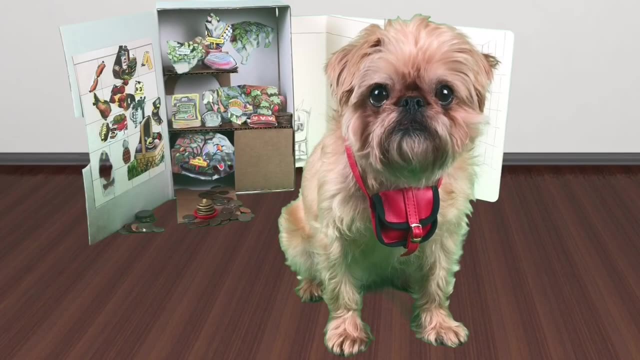 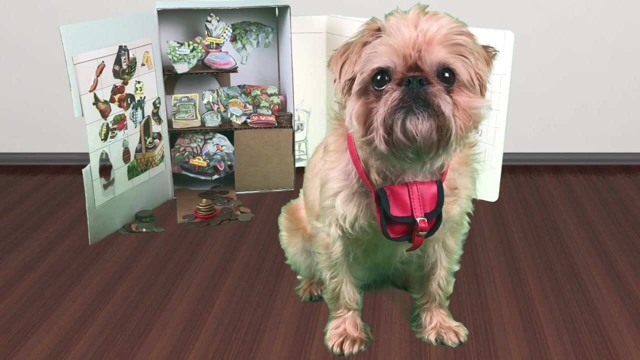 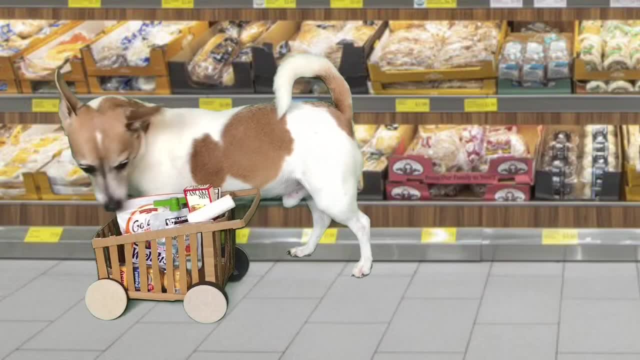 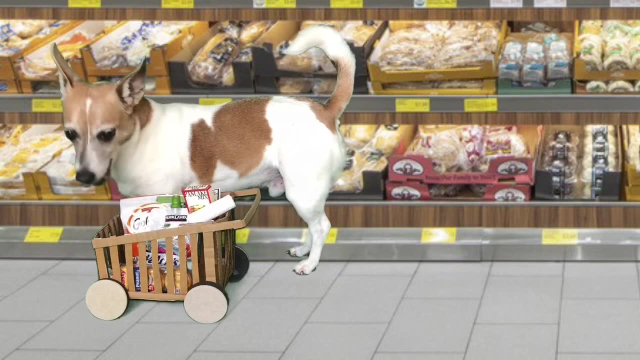 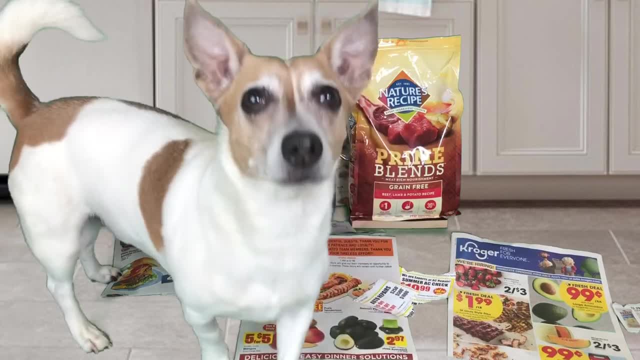 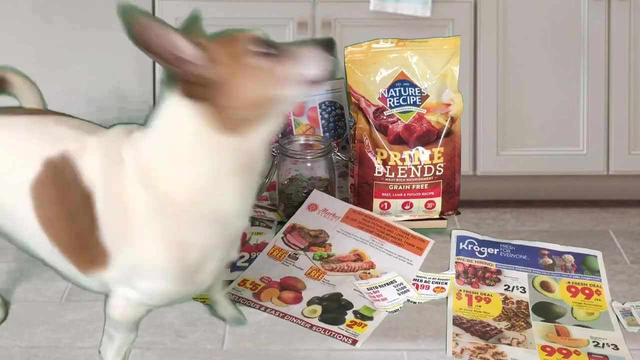 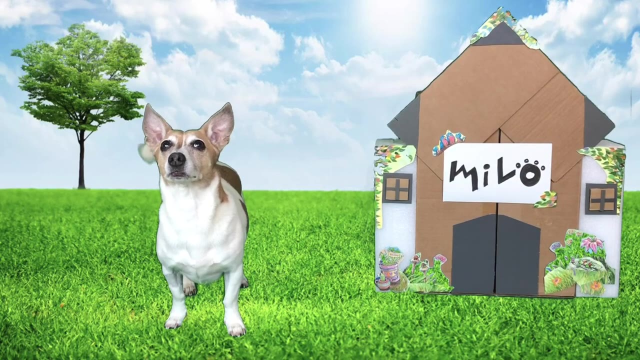 save even more money the next time he goes shopping. Milo, I can see your money jar. What are you saving for? It must be something special. Milo, you bought a house. You are an excellent saver. Can we see the inside?